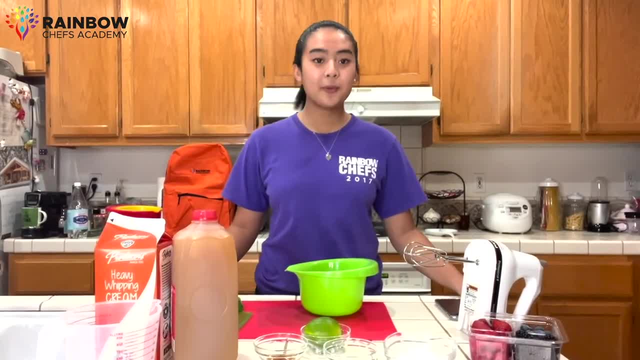 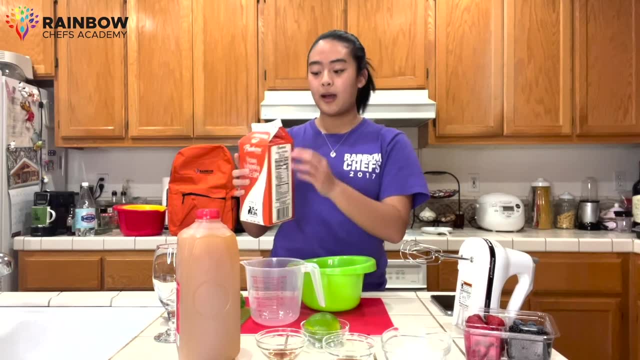 To start our daddy-off. we're going to start off with making our fresh whipped cream. So we're going to grab our heavy whipping cream along with our liquid measuring cup. We're going to pour about one and a half cups in, And then we're going to pour it into our medium-sized mixing bowl. 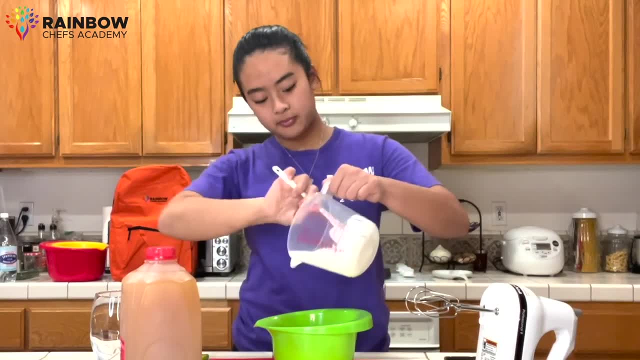 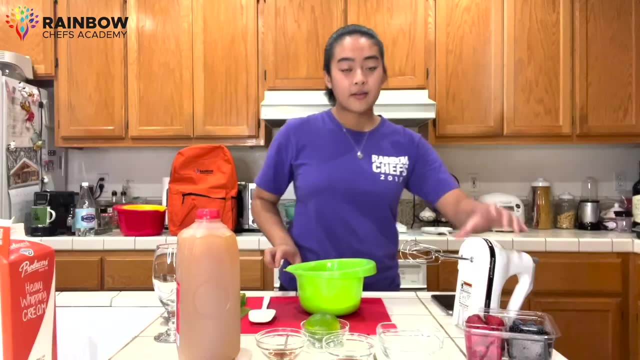 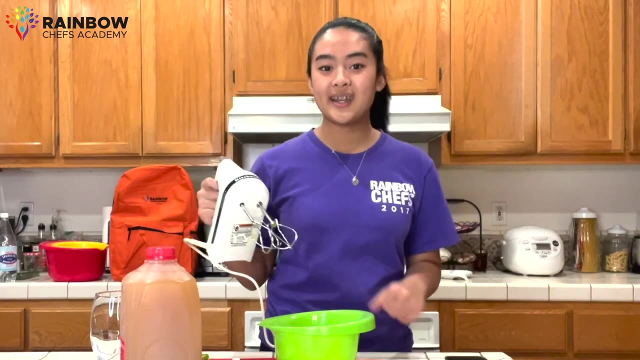 You can use your spatula to empty it up. Now we're going to add in our sugar. This is about one-third cup. From there, you're using your hand mixer. We're going to now blend until stiff peaks form. Little chefs, if you need help, don't be afraid to ask your parents. 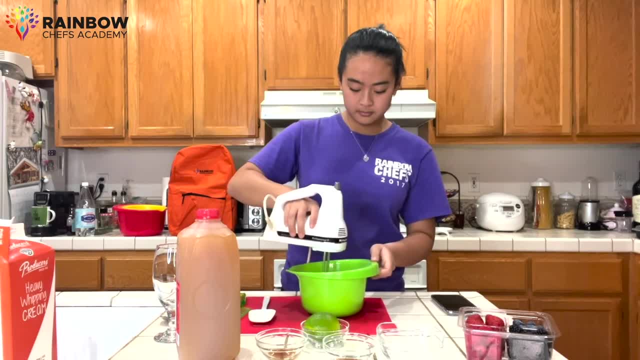 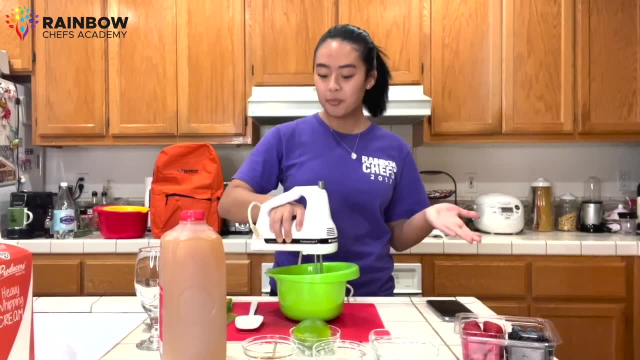 So, without further ado, let's blend. While we're using our hand mixer, we are whipping a bunch of air into our cream, which makes whipped cream. You can also use a whisk or a hand whisk to mix your own whipped cream by hand. 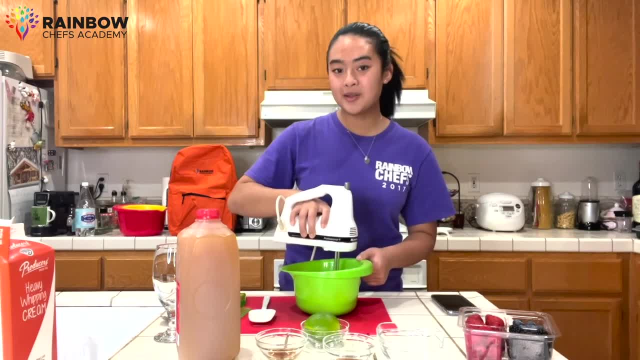 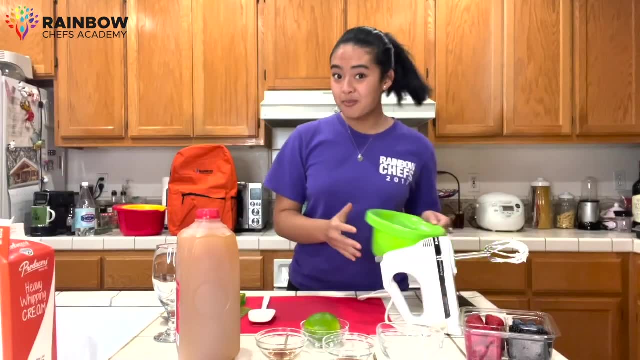 but it does take a little bit longer. Feel free to rotate the bowl to get all around the bowl. Are you wondering what stiff peaks look like? Well, this is what it looks like. It's until the whipped cream can hold its form. 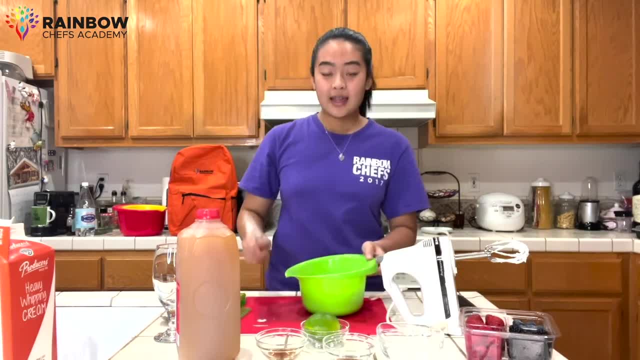 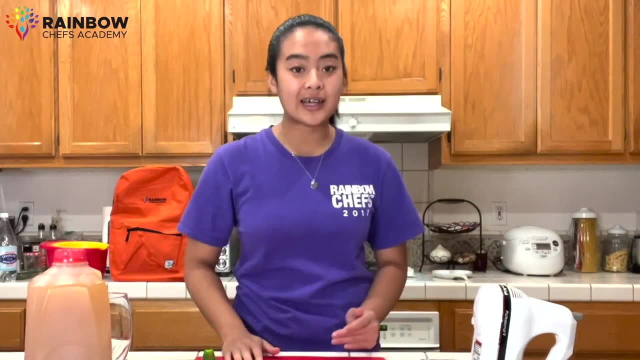 Mmm, this looks so good. Now I'm going to give it a quick little mix with my spatula. From there, we're going to put this aside. Now that we've put aside our whipped cream, we're going to now start slicing our berries. 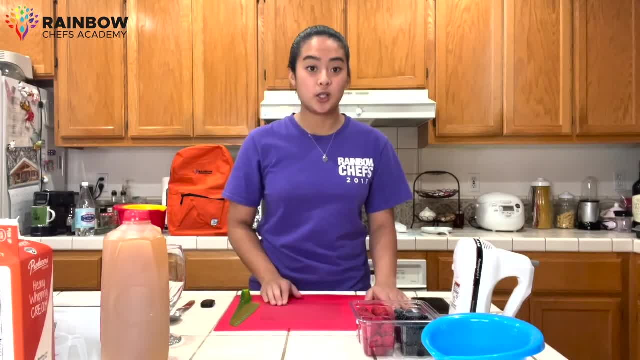 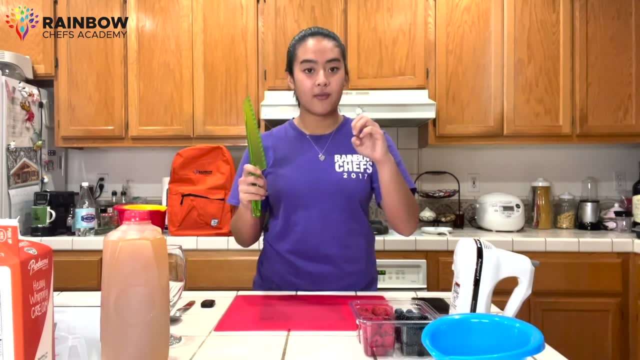 So whenever we cut anything in the kitchen, we always want to make sure to hold the claw fingers, So that way we avoid cutting our fingers while using our sharp knife. While holding a knife as well, we would like to use the pinch grip. 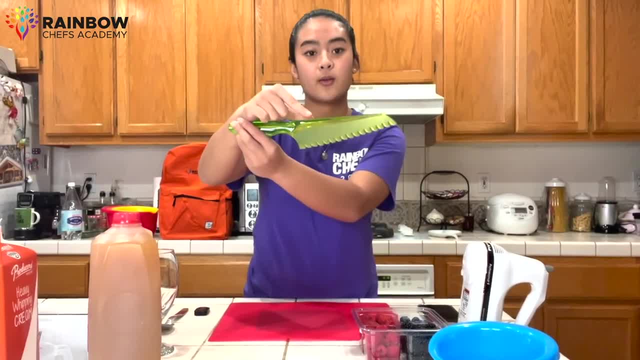 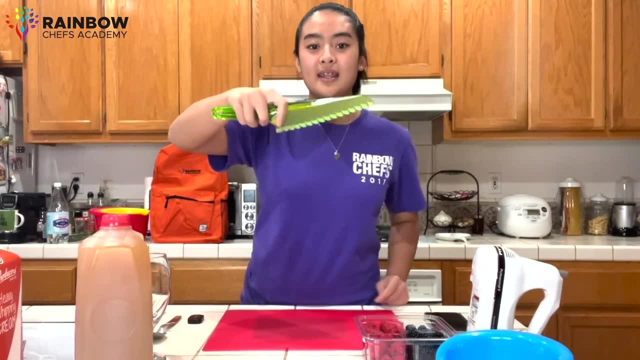 So if you use your pointer finger and your thumb, you're going to pinch the bottom half of the knife and the rest of your fingers- you wiggle them around- are going to grab the handle. This is called the chef's pinch grip. 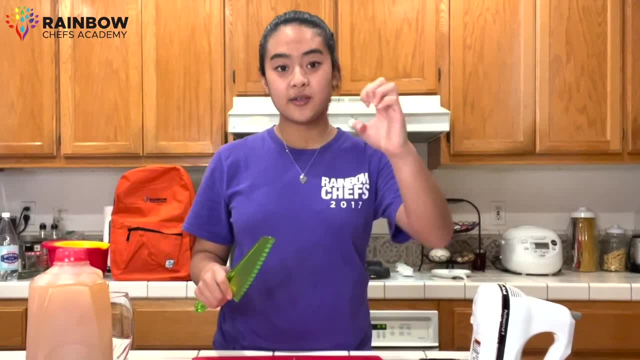 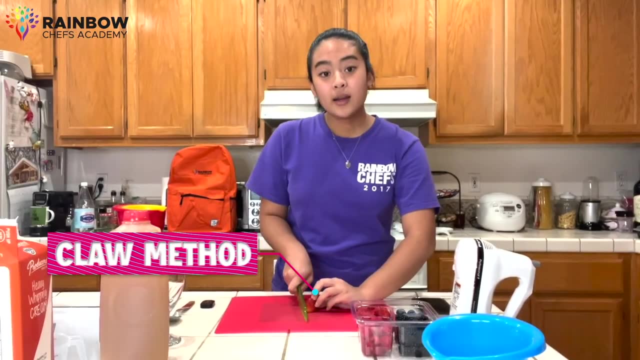 Like I said, we're going to grab a strawberry and using our claw, tucking in all of our fingers, just like this, we're going to hold our berries still, so that way it's easier for us to cut. When cutting, we also want to use a wave motion. 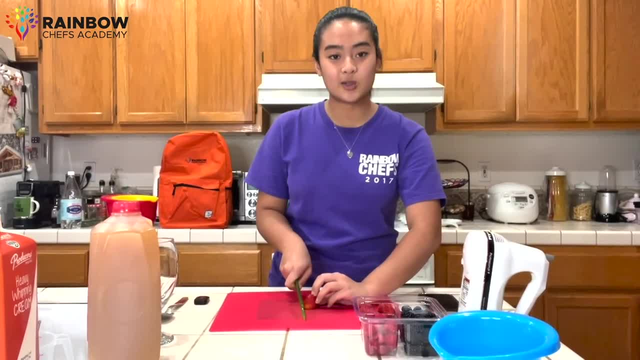 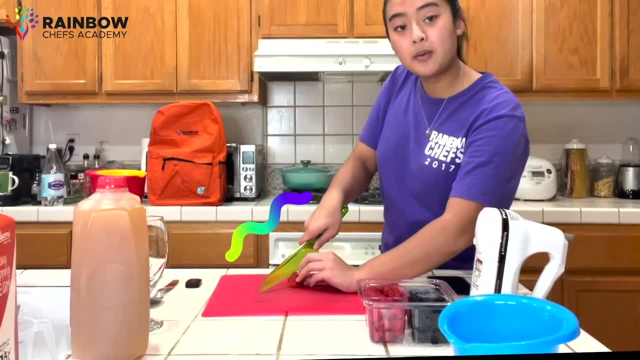 so that way we go through all of our berries, That way we go through all of our ingredients nice and smoothly. So we're going to lift, keeping the tip of the knife on the board, We're going to place the middle part of the knife on the strawberry and wave down. 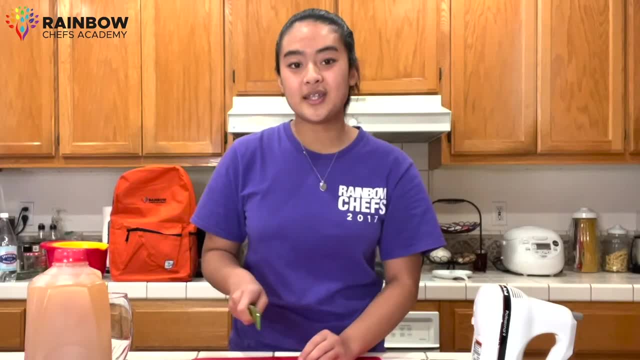 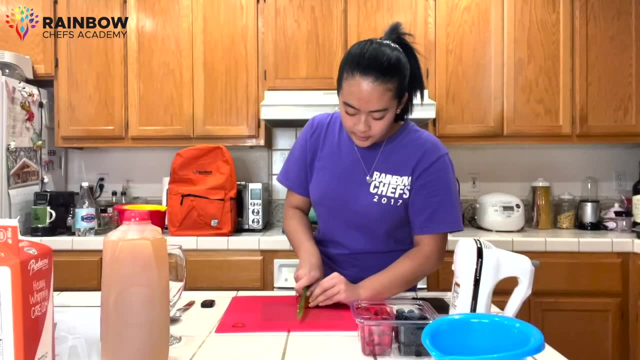 And there you have it, a nice sliced strawberry. I'll do this a few more times so you can do it with me Using the claw grip again, wave motions, cutting our strawberry nice and thin For the blackberries, we're simply going to cut them in half. 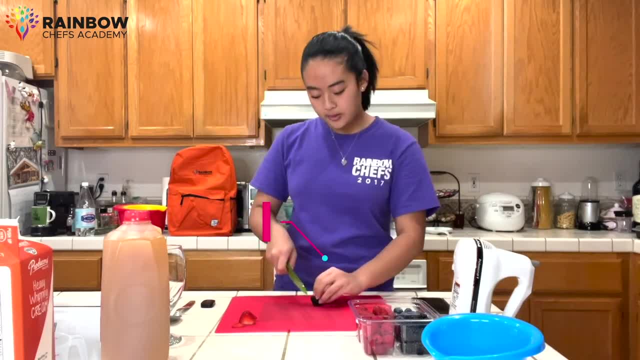 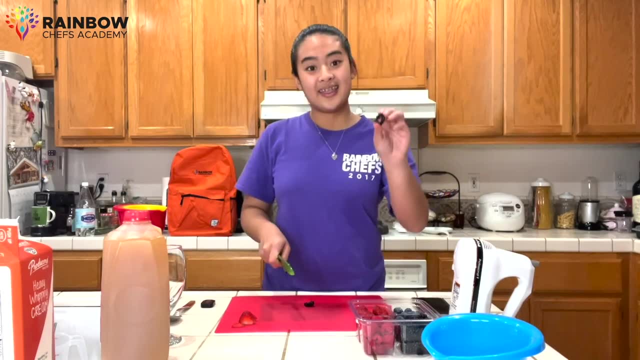 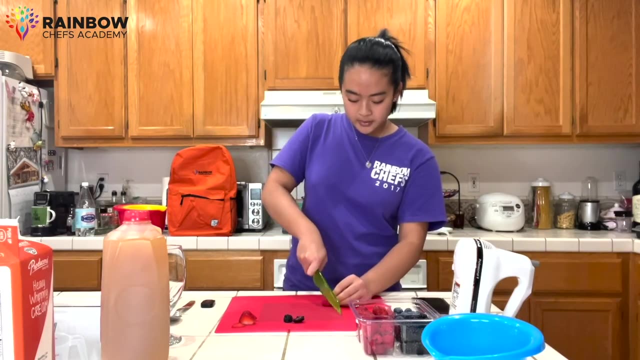 No need to slice them. So, again, using the claw wave motion and our pinch grip, nice and slowly slice down. There you go. there goes the blackberry. We're going to do the same for the raspberry. Claw, pinch grip wave, perfect. 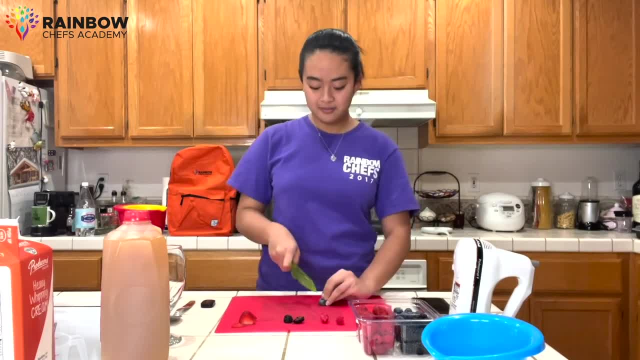 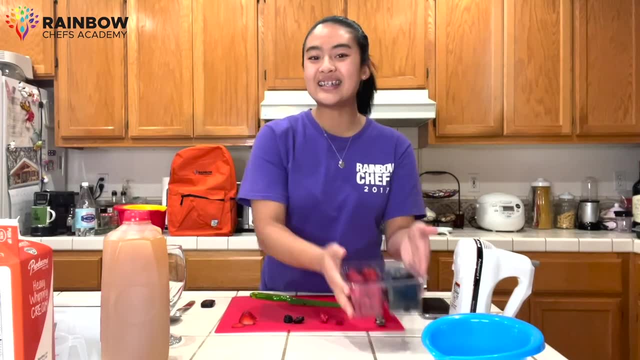 And our blueberries: Pinch, grip, claw, wave, motion, perfect. And there you go. Continue this for the rest of your berries. Now that we've finished cutting our berries, I'm going to top it off with some lime juice. 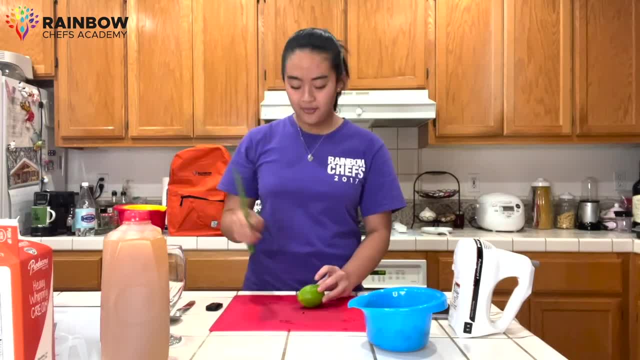 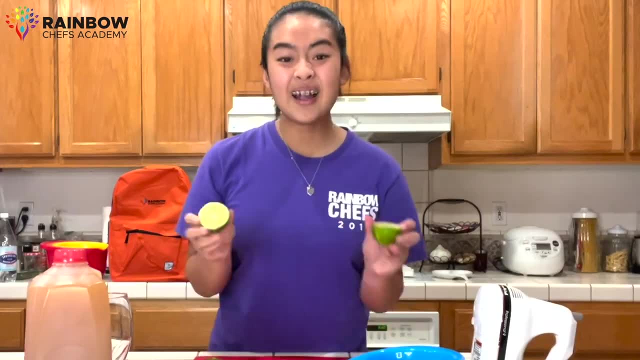 So I'm going to grab our lime using our knife and slice it in half, Again using our claw, our pinch grip and slicing very slowly. Look how pretty. From there we're going to squeeze a little bit of lime juice on top of our berries. 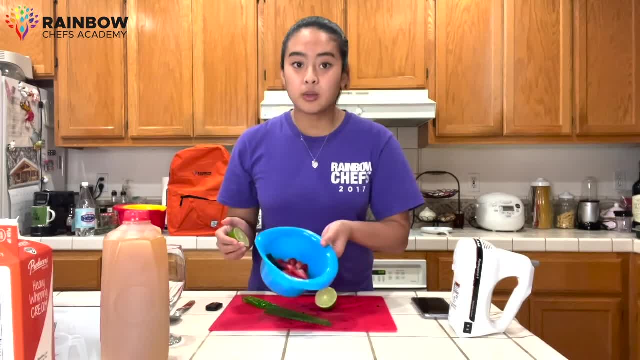 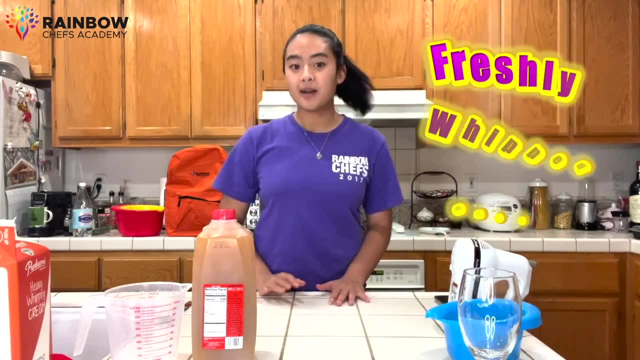 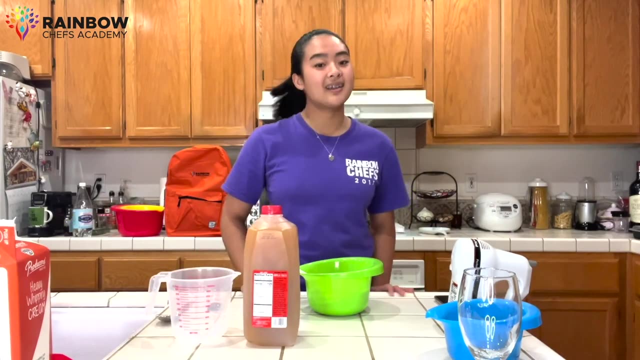 That way they don't get bad and they keep their gorgeous color. And now we're going to put our berries inside. Next, we're going to grab our freshly whipped whipped cream, along with our apple juice and our liquid measuring cup. We're going to measure at exactly two-thirds cup of apple juice. 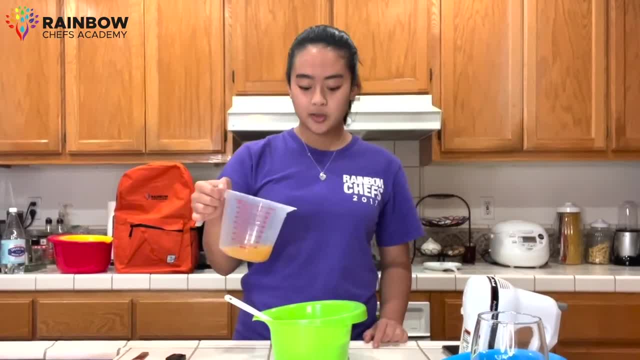 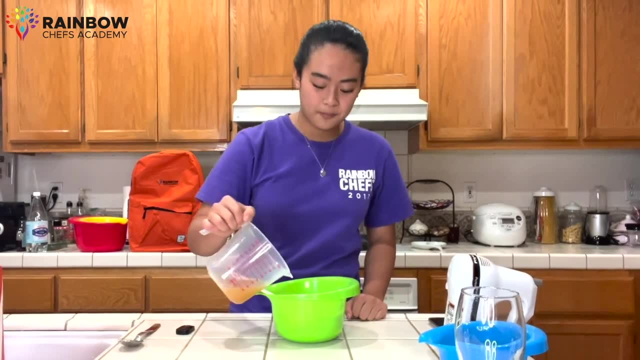 From there, we're going to slowly add little additions of the apple juice into our whipped cream. We're going to want to fold it in slowly, And I will go over what folding means in a second. So pour in a little bit of apple juice. 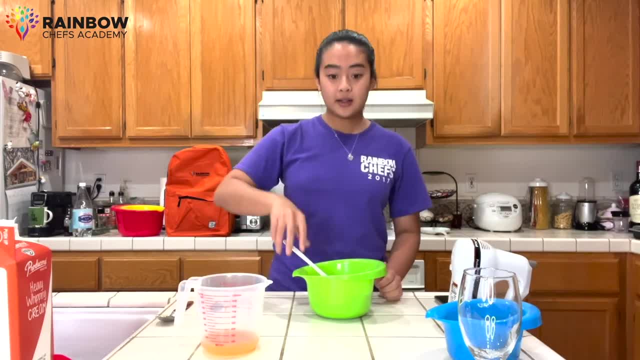 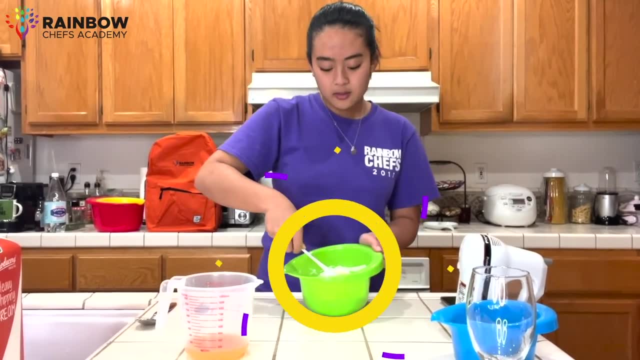 Stop Put it to the side To fold. we're going to grab a spatula with our overhand, just like this in our bowl. We're going to go around the bowl and make a circle and fold right on top. So again, we're going to go around the bowl and on top. 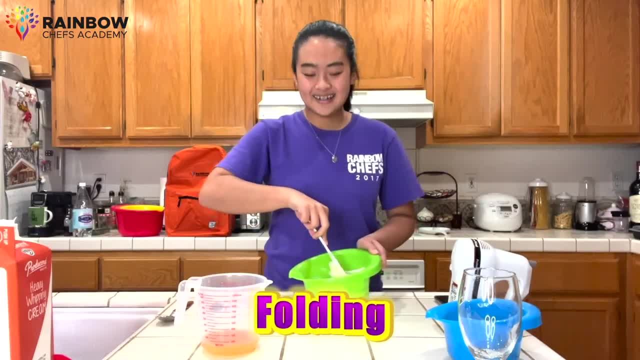 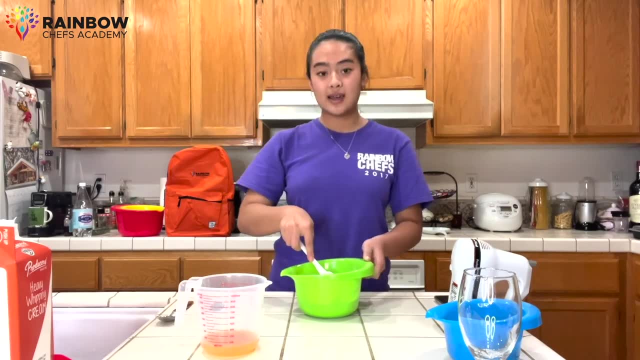 Around the bowl and on top. This is called folding. Keep adding apple juice until you run out. Folding allows the air to escape very slowly, so that way our whipped cream still tastes nice and fluffy, and it still tastes just as good.